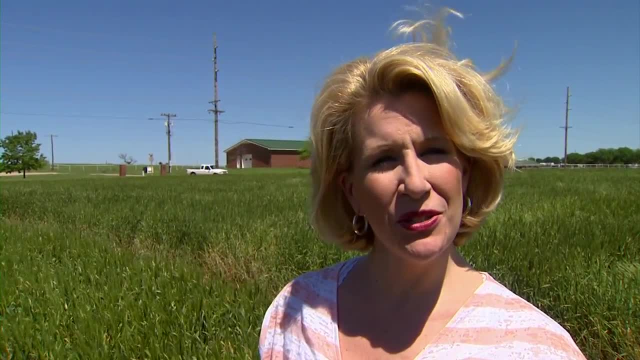 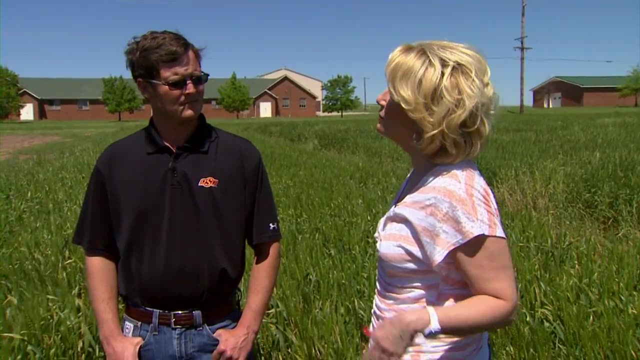 With the recent rains that we've had this spring, now's a good time to assess your soil for compaction. Joining us now is Jason Warren, our soil management specialist. And Jason, why now this year? Well, a lot of times people ask me about compaction and they generally wait until. 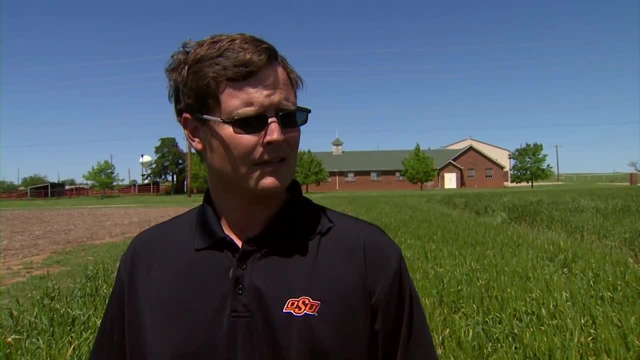 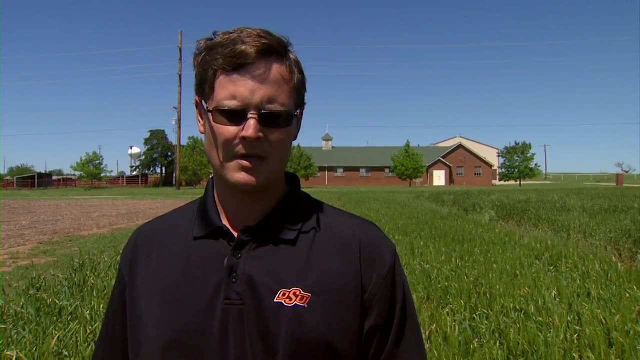 the summertime- because we're particularly wheat farmers are off, You know they're not busy harvesting or planting or managing the crop, They're just trying to get ready for the falling crop. And the summertime is probably one of your worst times because our soils tend to be. 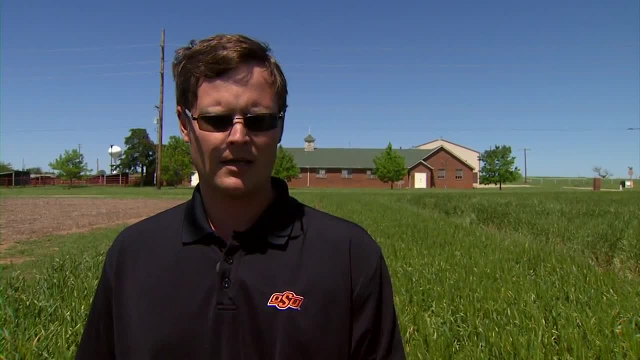 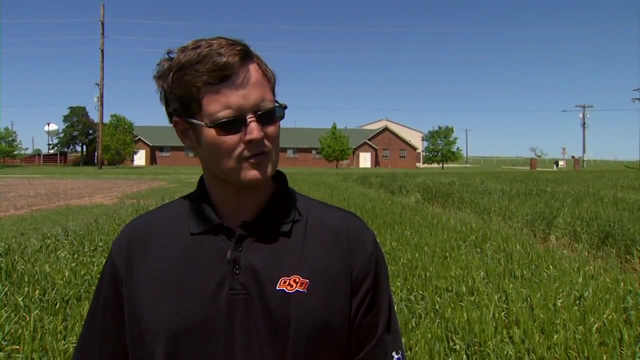 dry. But now that we've had all this nice rain in a lot of the state- and then hopefully we'll continue to get some nice rains throughout the rest of the spring, our soils will be well-suited to assess compaction, Because when we look at compaction we don't want to look at dry. 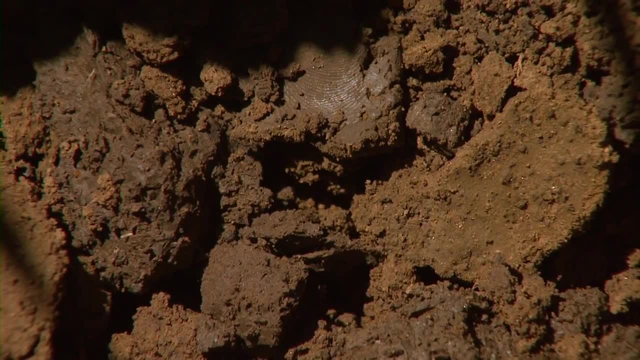 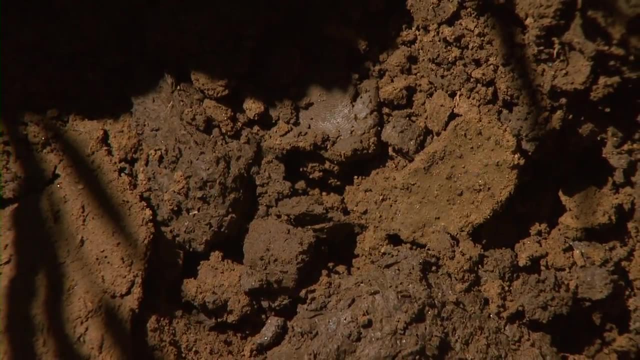 hard soils. We want to look at our moist soils and see if, when under moist conditions, is that compaction sufficient to limit root growth. And so when we look at compaction, we can look at what's going on in the soil. We can look at what's going on in the soil. 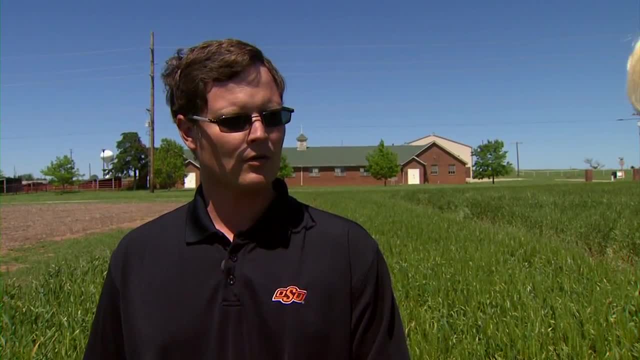 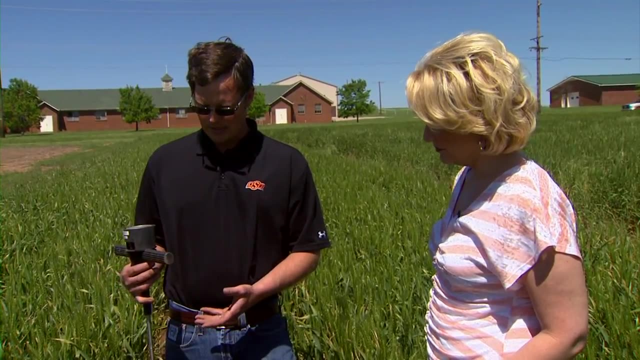 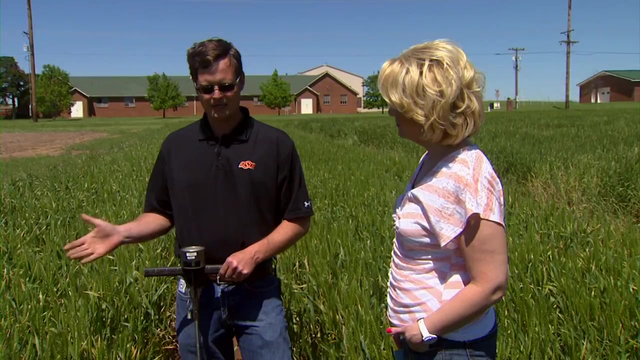 We can visually observe, you know, horizontal layers or horizontal root growth, Or we can use something like this as a penetrometer, Or even- you know this is a $200 deal- You could just have a steel, a pointed steel rod with a T-handle on it and make your own penetrometer and kind of feel. 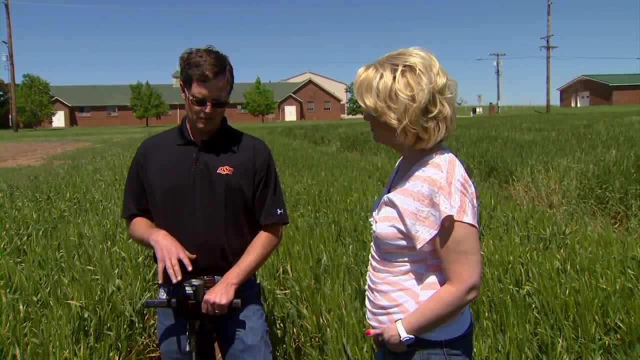 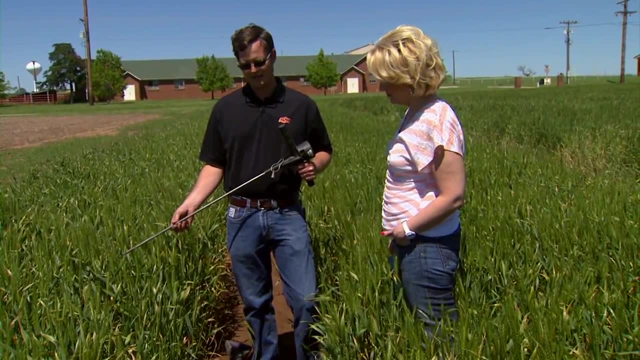 around for dense layers in the soil, But anytime you do any kind of penetration resistance is what they call this. we certainly want to do it when the soil is wet, Because as soon as this hits the ground, just like anything else, it's going to get wet, And that's what we want to do. 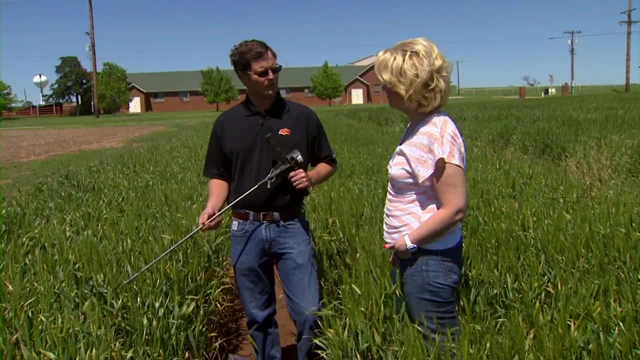 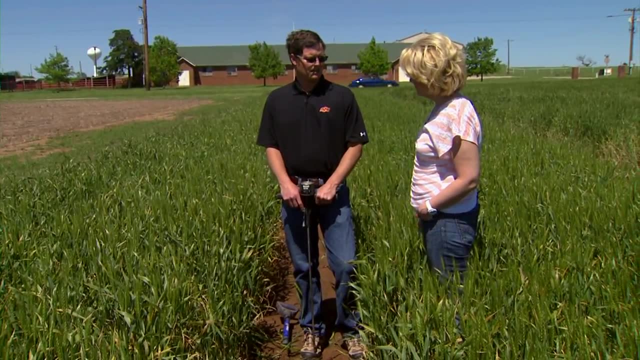 Just like anybody knows from digging post holes or any kind of hole, dry soil is hard and roots aren't going to go through it regardless, So we want to do it when the soil is wet, like it is today here in Stillwater. Okay, You kind of dug a little hole here. 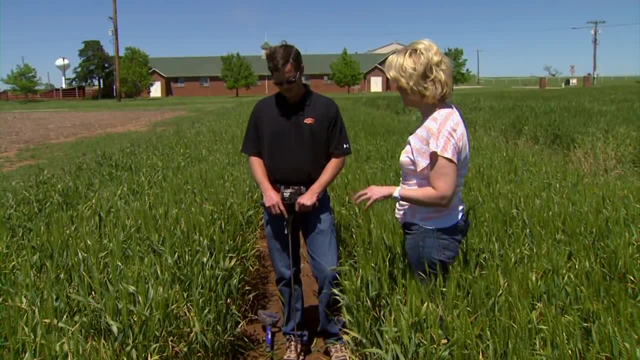 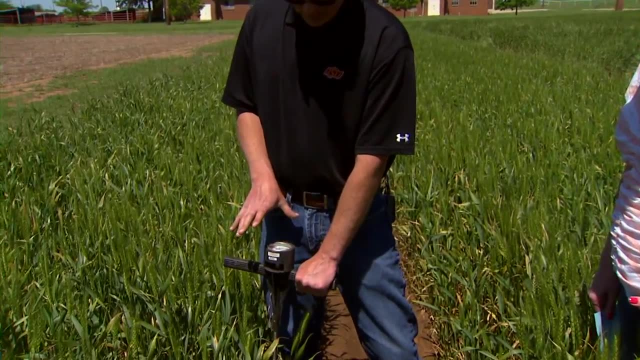 and did a test. What kind of things did you find with this particular soil that we know has gotten lots of rain lately? Well, first thing we do is we can push it down, And when you're doing, whether you're using a steel rod or a penetrometer like this, 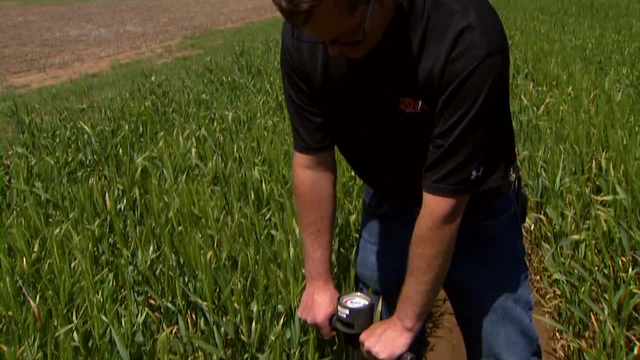 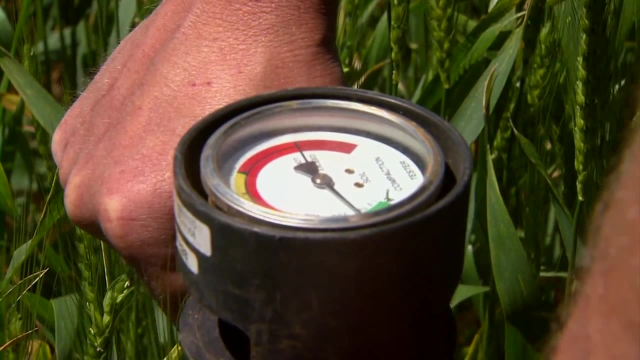 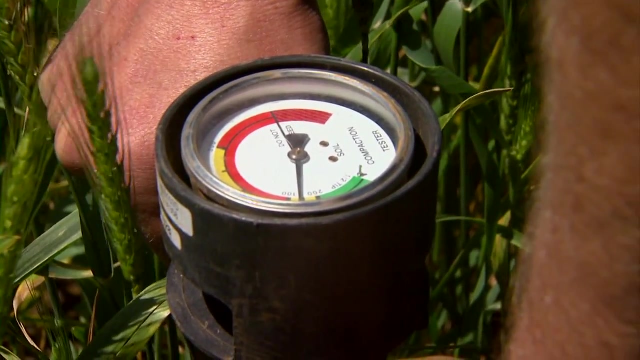 you want to slowly push it down and slowly push it down until you start to see resistance And essentially the resistance of a soil is more where it stops to move downward. You'd look at the reading and you can keep pushing it, And we want to on a penetrometer. 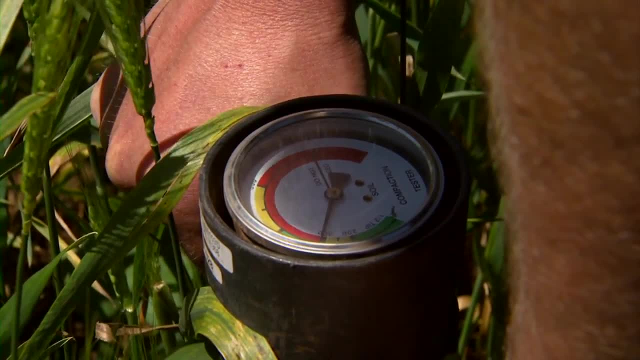 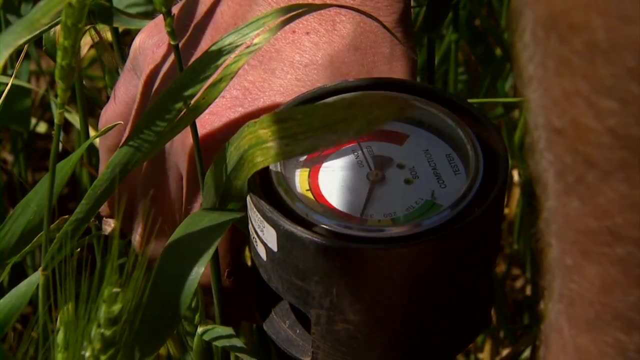 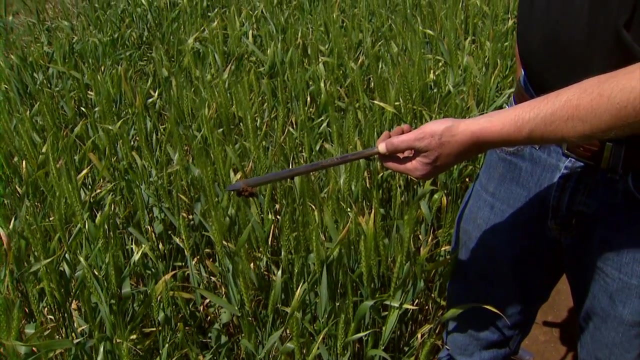 if the penetration resistance is greater than 300 psi, then we can limit root growth. And what I find is about: I can get penetration resistance there of around 300, and that's about six inches on my rod here, And so what I've done is dug down there to kind of get an idea what that might be. 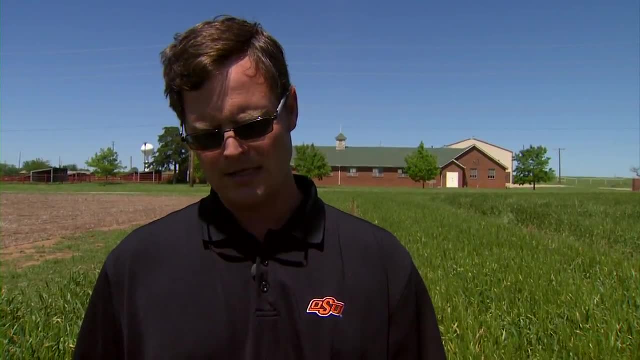 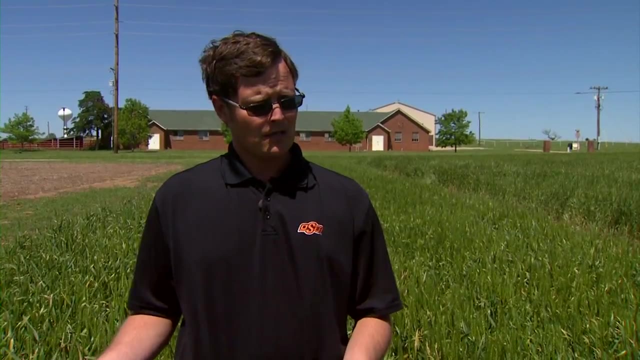 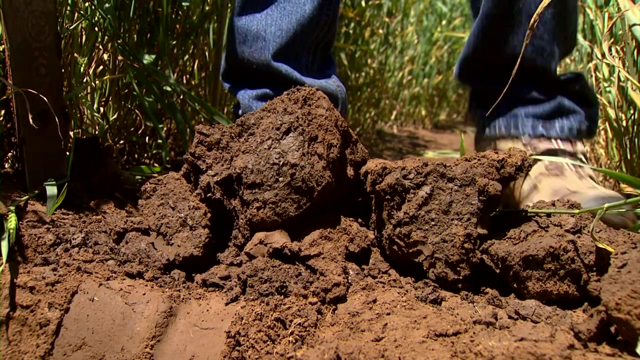 Because you can have. you know, plow pan would be common at six inches. Clay pans could also be common there. Had we not had six inches in the last two weeks here we'd possibly have dry soil, But what we find is an increase in clay content. You see, this pad is nice and shiny. 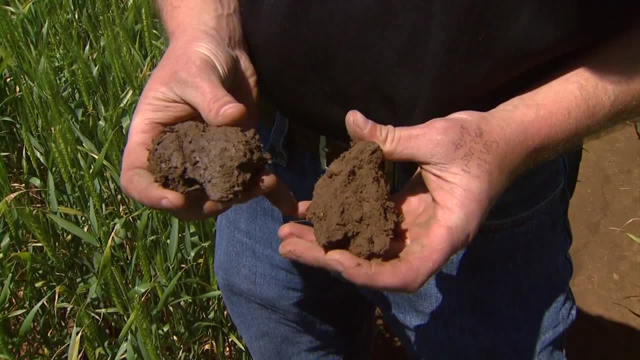 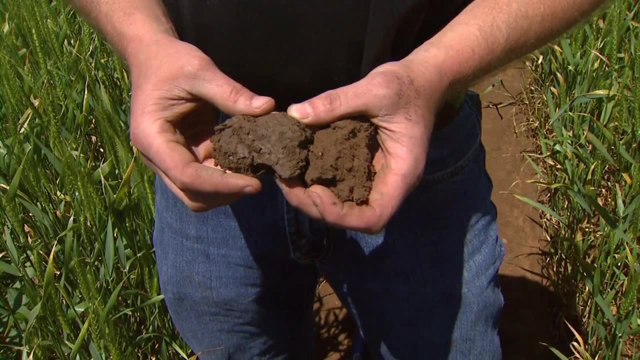 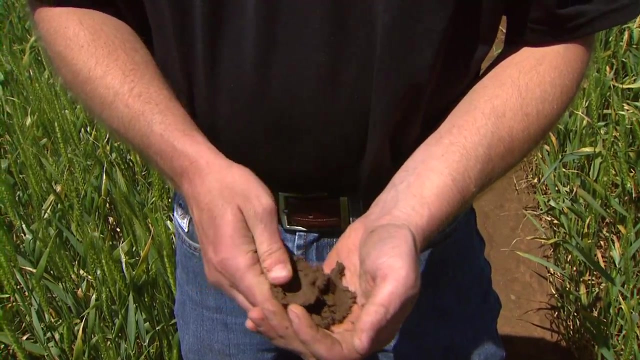 whereas this one's kind of dull. It's got sparkling sand grains in it, but the surface isn't shiny. Well, from visually, that shiny surface tells me there's more clay in it than what's in the surface. And then when you start to put it between your thumb and finger, 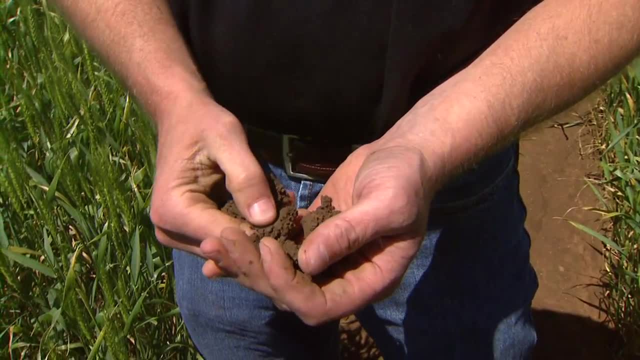 you can see it sticks together real readily and starts to kind of shine, And it's more the feel than the look. And then, when you start to put it between your thumb and finger, you can see it sticks together real readily and starts to kind of shine, And it's more the feel than the look. 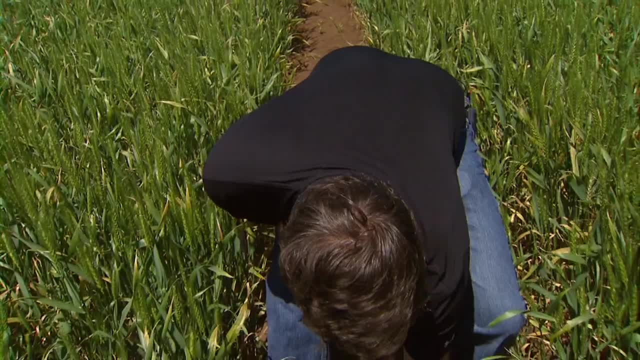 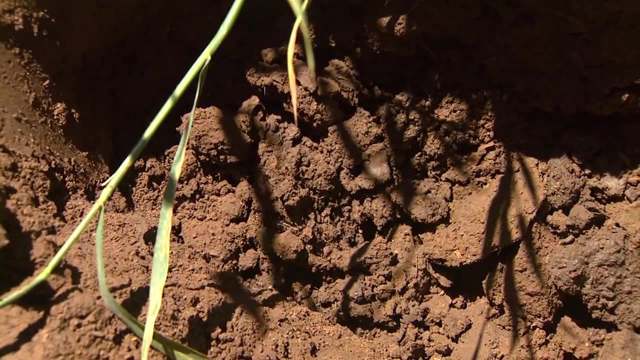 That look is what you can see there on TV, And so what we know is they're about six inches. We may have a plow pan there, because this is cultivated cropland, but we also certainly have an increase in clay. that is has got something to do with that penetration resistance. So then the 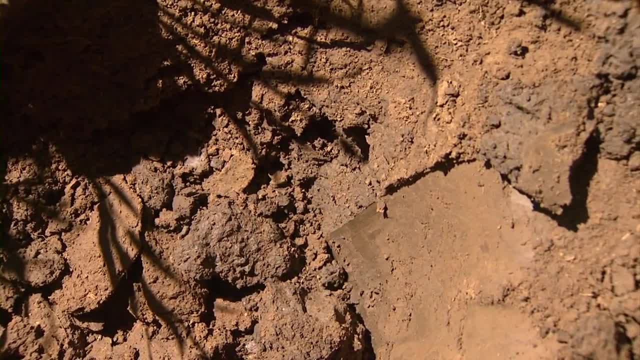 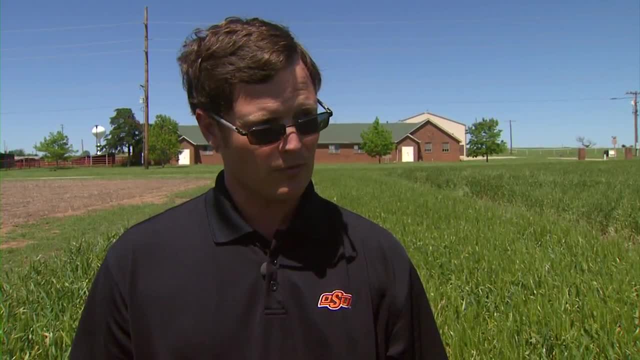 question becomes: do we want to try to physically remove that compaction On a heavy clay soil or subsoil like that? it's gonna cost you a lot of money to run a deep ripper through it, And so I would probably say no. I'd let nature take its course, and throughout the summer the soil will shrink and expand and break apart and probably do just as well as running some kind of heavy equipment through here. Okay, and for wheat farmers you can kind of do, and canola I'm sure kind of do this after harvest as well. Yeah, in fact, the nice thing about wheat and canola is as they dry.